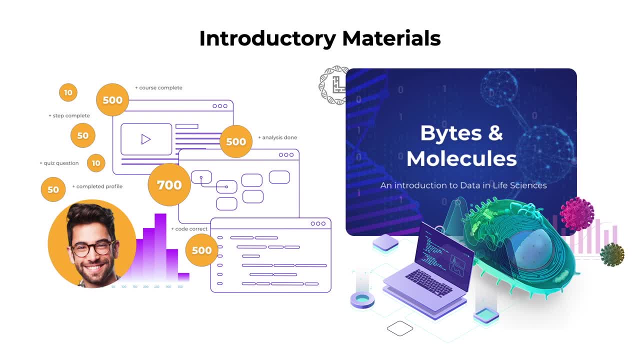 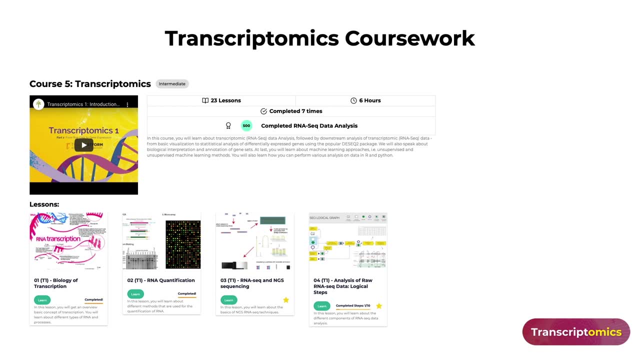 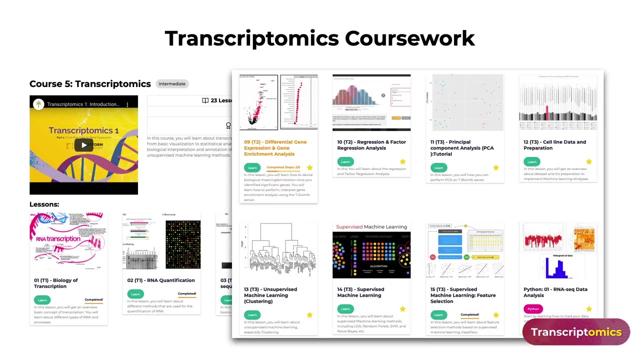 overview of important research topics and applications of bioinformatics. for a novice, The main transcriptomics module will provide you with in-depth materials on specific challenges for RNA-seq data analysis, both in small datasets and large-scale studies. The theoretical training will be supplemented by exercises using the T-by-Info analysis platform for processing. 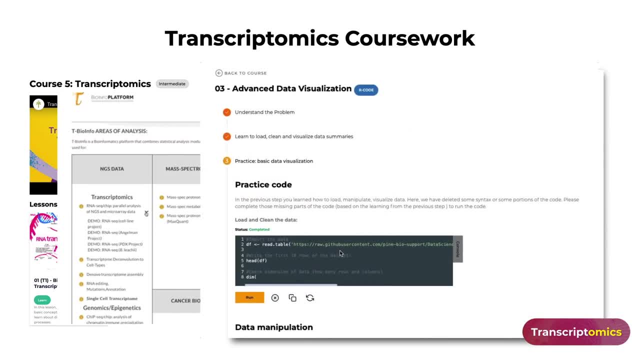 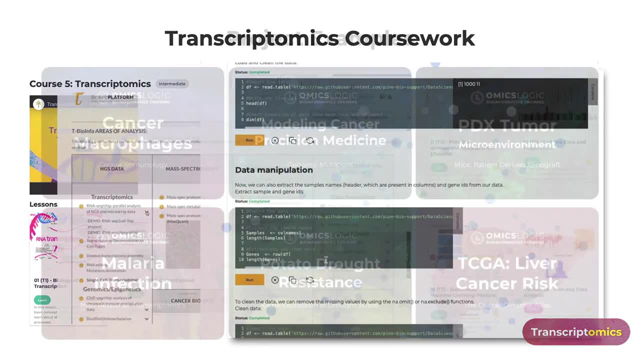 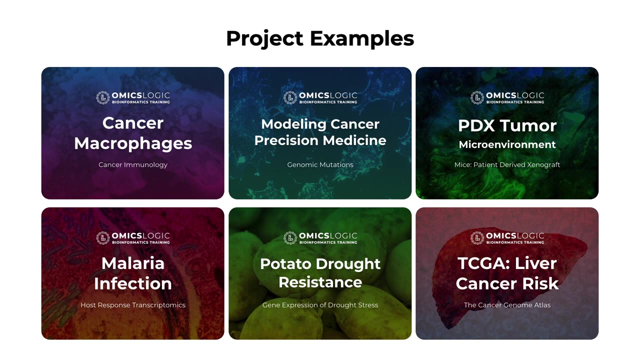 assignments and optional coding exercises, which can be completed in R or Python on your computer or using our online coding environment. In addition, you will find a range of project examples to see how such techniques are used in oncology, immunology, infectious diseases and agriculture. 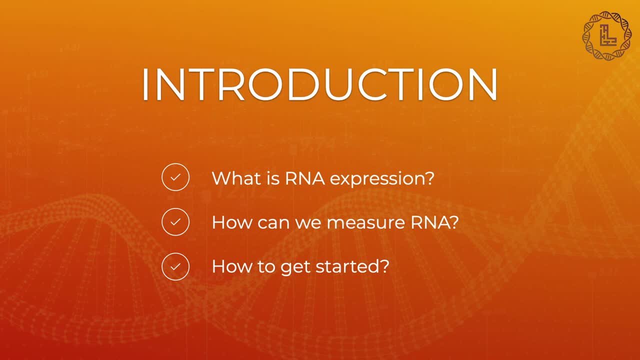 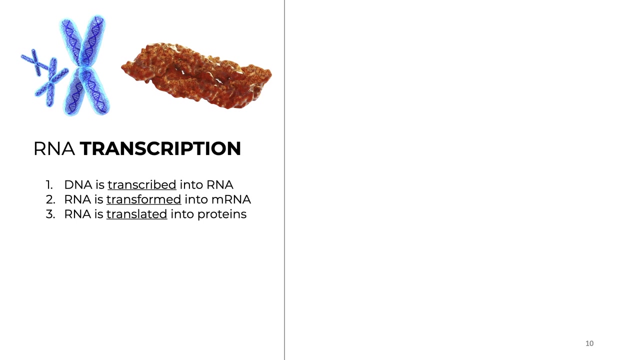 Today we will start with an introduction. What is RNA expression, how can it be measured and what are some of the technical steps to get started with next-generation sequencing data analysis for gene expression quantification? The process of RNA transcription is key to determine the cellular phenotype. 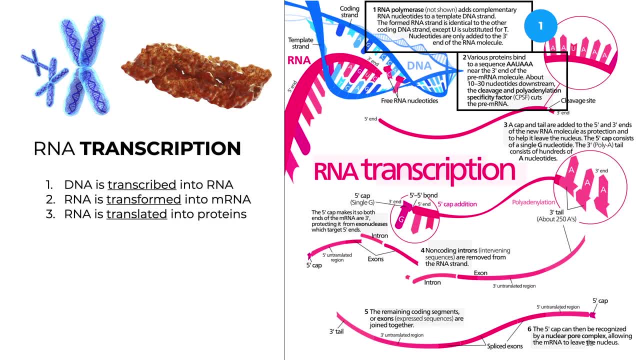 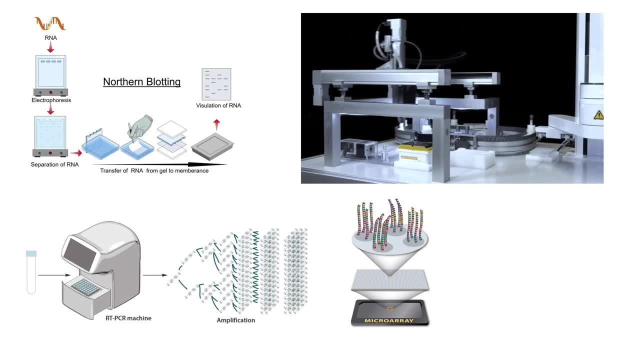 It kicks off with RNA polymerase, adding complementary nucleotides to a DNA template strand. As a result of modifications at all of these steps, the cell phenotype is determined, resulting in over 200 different types of cells in the human body. These technologies developed over time, becoming more and more sophisticated as a result of. 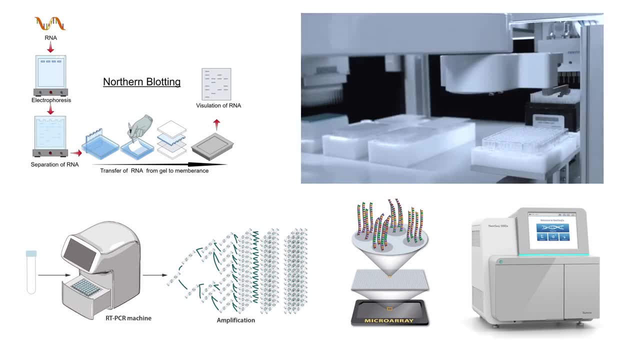 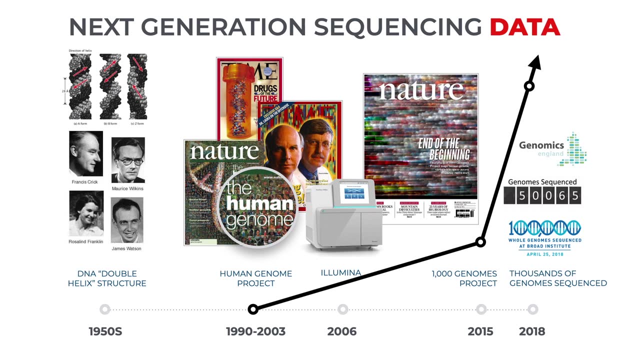 automation, refinement of the technology and a greater understanding of the underlying biology. The R&D studies are a powerful tool to build a more robust and more comprehensive world's understanding of the underlying biology. Today, the cost to sequencing DNA puts these technologies a full genome is already less than a thousand dollars, And there's an ever-increasing number. 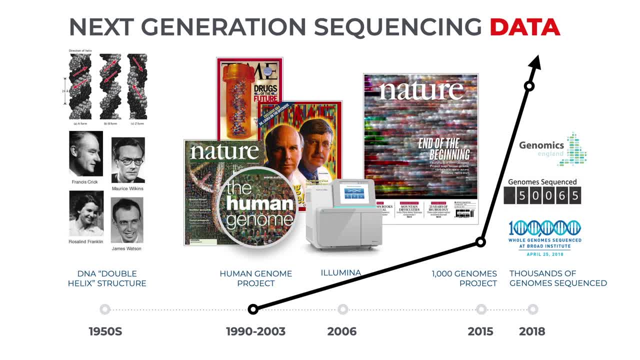 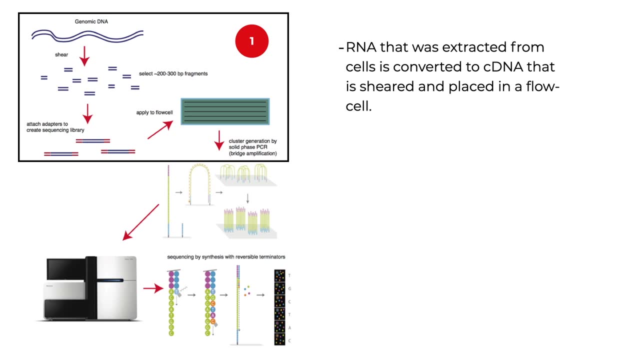 of genomic, transcriptomic, proteomic and metagenomic data sets available for the public to use that describe subcellular processes with highly detailed digital data. First, RNA that was extracted from cells is converted to cDNA that is then sheared and placed in a flow. 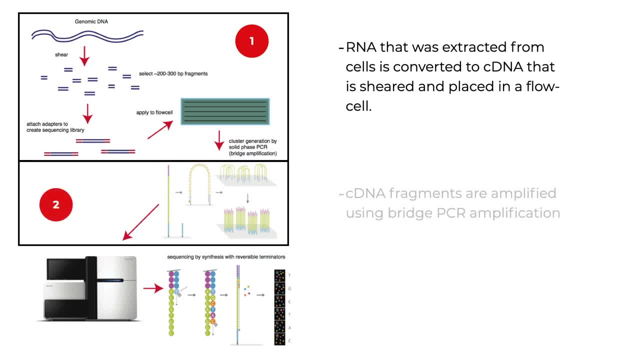 cell. Inside the flow cell, the cDNA fragments are amplified using bridge PCR amplification and the flow cell is inserted into the sequencer. This machine uses image analysis to capture each letter in the flow cell by analyzing visual patterns and converting them to a sequence.